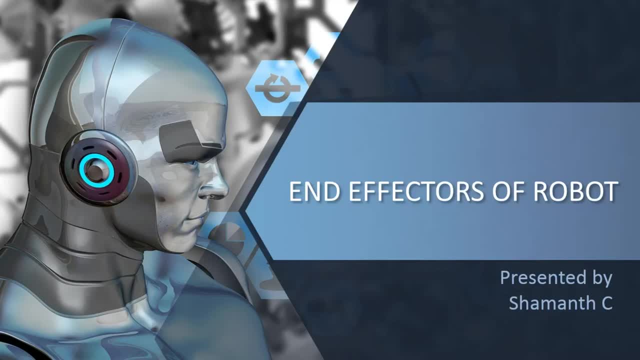 Hello, my dear learners, Welcome to my lecture series on robot technology. In this lecture I will be explaining about end effectors of a robot. This lecture is presented by me, Samant. You might have seen my previous video lectures wherein I have explained about the robot: specification, physical configuration of a robot, anatomy of a robot, everything. If you have not seen, do click on the link which is on the top right corner and then you can see my previous video lectures. 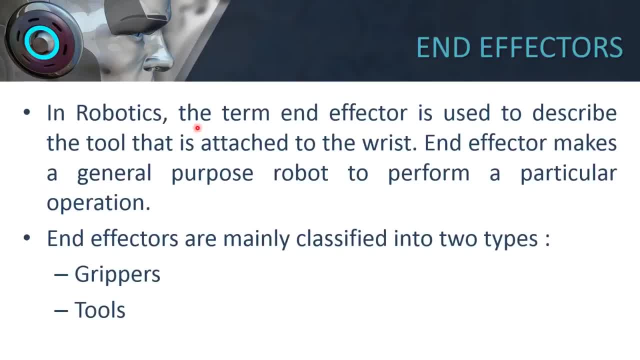 So let us begin today's lecture. In robotics, the term end effector is used to describe the tool that is attached. You imagine holding a pen in your wrist: Pen is the end effector. You imagine holding a spoon in your wrist: Spoon is your end effector. 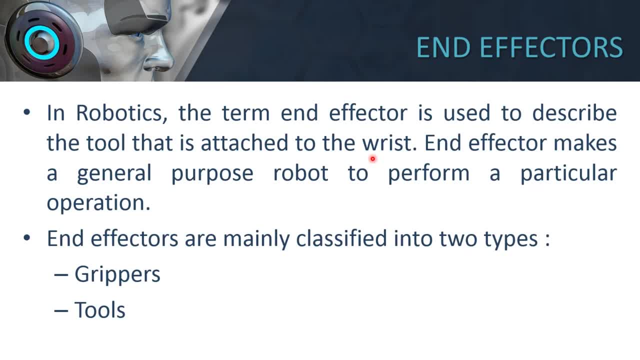 So it is used for making a general, a particular operation. Say, why do you use pen To write? Why do you use a spoon To eat? So that is how you define the end effector. as There are different end effectors for a robot as well, We will see what are those end effectors. 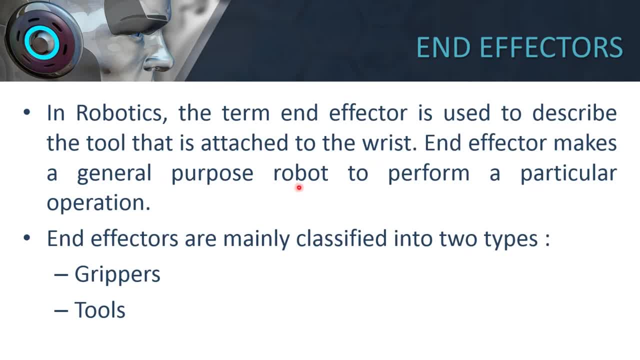 End effectors generally makes a general purpose robot to perform a particular operation. You can make the robot to perform the operation according to your instruction by the help of the end effector. There are two types of end effectors: One is grippers, The other one is tools. 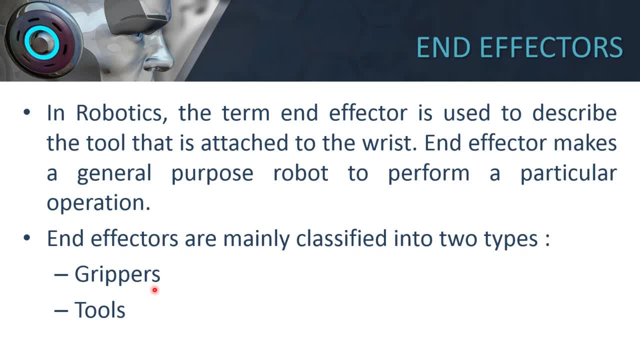 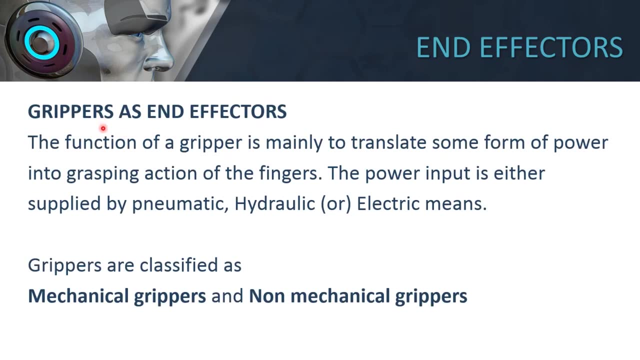 Grippers are mainly used to grip certain products or any part or a material, whereas tools are used to perform a specific task. So we will see that. We will see what are they? Grippers as end effectors. When you are using grippers as an end effectors in a robot, the function of the gripper is mainly to translate some form of power into grasping action. 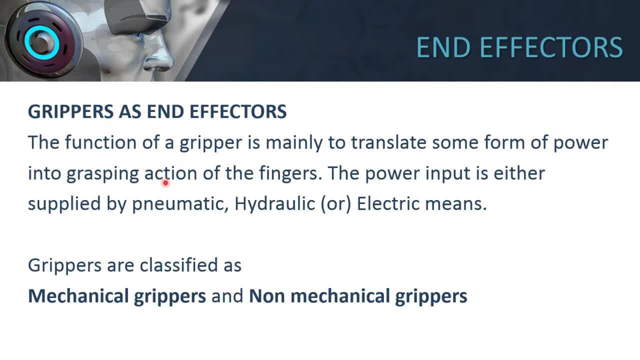 Say, for example, you want to drink Pepsi. When you have to drink a Pepsi, you want to grasp the can of Pepsi in your hand and help yourself to drink it. If you have to take it to mouth, then you have to grasp that can of Pepsi. 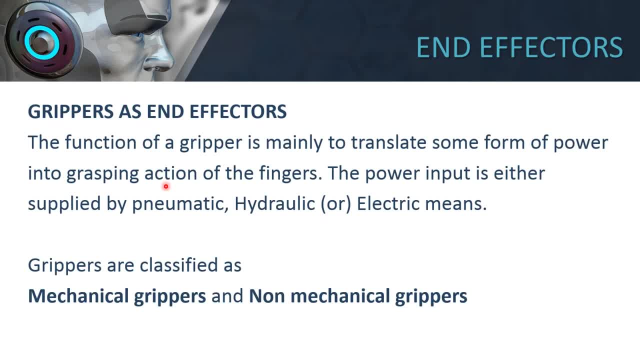 And then bring your arm up near to your mouth and then you have to pour the Pepsi in the can into your mouth. The same way, if a particular material or a part has to be grasped, then a robot requires a gripper. It is used mainly to translate some form of power into grasping action of the fingers. 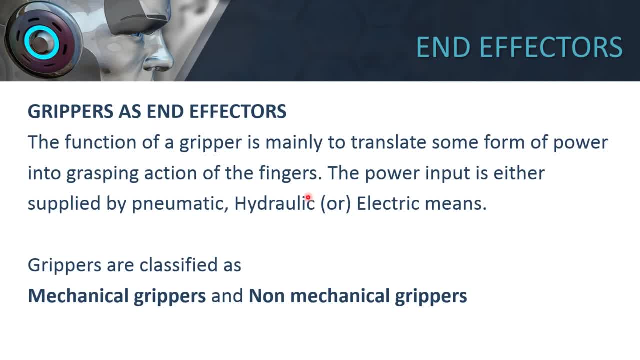 So there might be some power which the robot might be using. Some form of it will be used to grasp the object. The power input is either supplied by pneumatic, hydraulic or electric means. There are two types of grippers. One is a mechanical gripper. 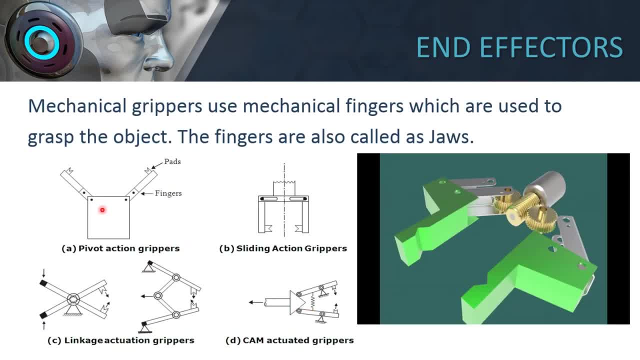 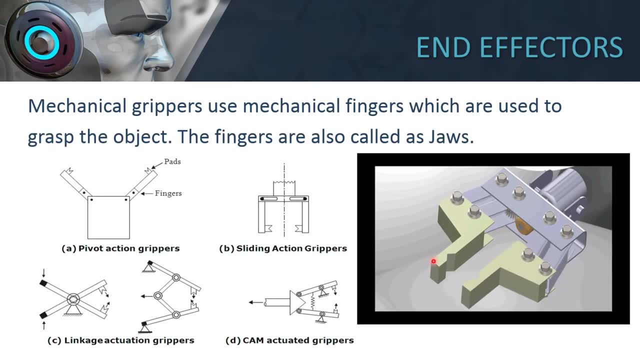 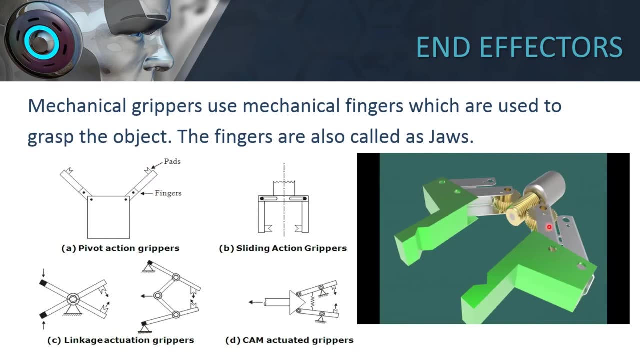 The other one is a non-mechanical gripper. So generally the mechanical grippers use mechanical fingers which are used to grasp the object. You can see the animation here. These are the mechanical fingers which is used, or which is with the help of the worm and the gears. 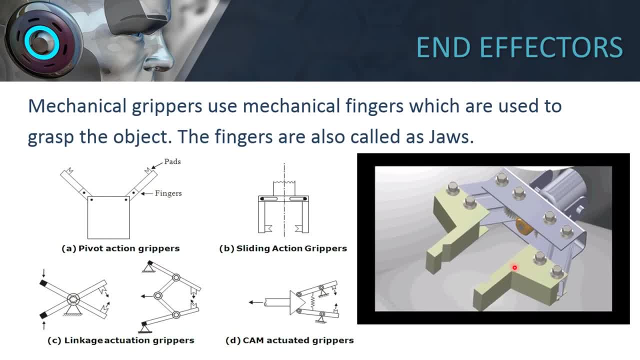 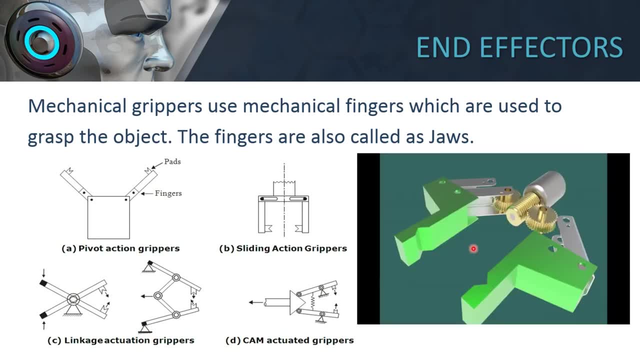 It can be operated Based on the operation, That is, by the help of a pneumatic drive or a hydraulic drive or a electric drive. It can be operated and the fingers can be brought in contact, So based on how much dimension the product is. 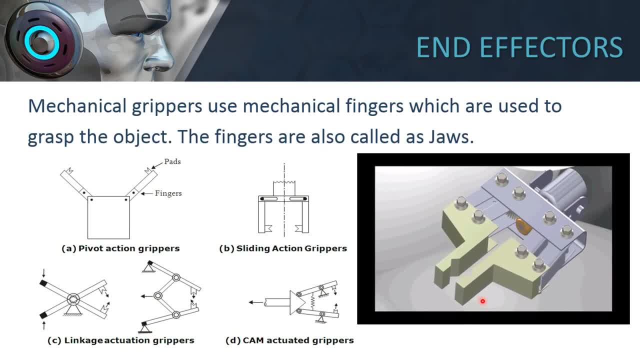 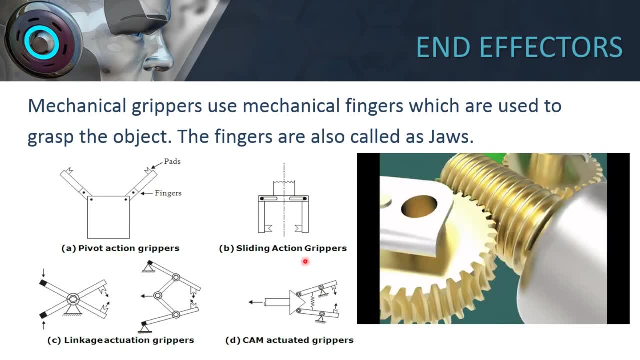 Based on that, it can sense and then it can grasp the object. There are different types of jaws which are available: Pivot action grippers, sliding action grippers, linkage actuation grippers and then cam actuated grippers. This is a gear actuated gripper. 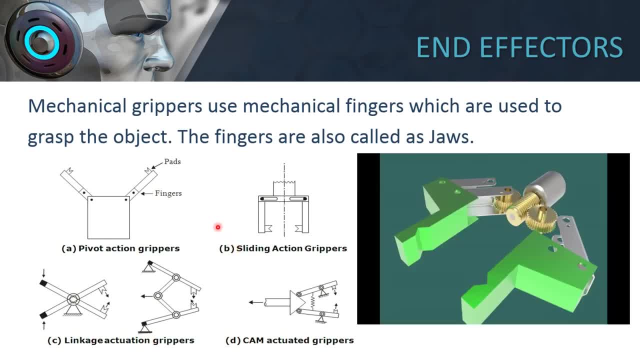 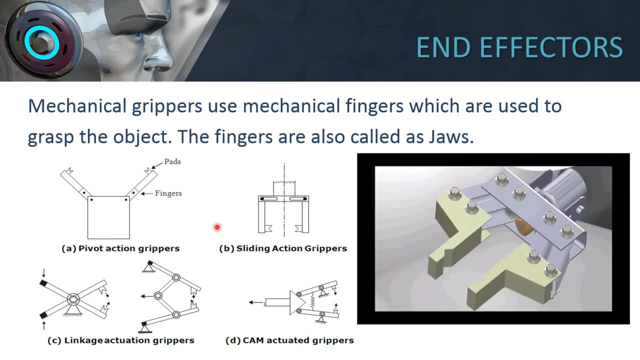 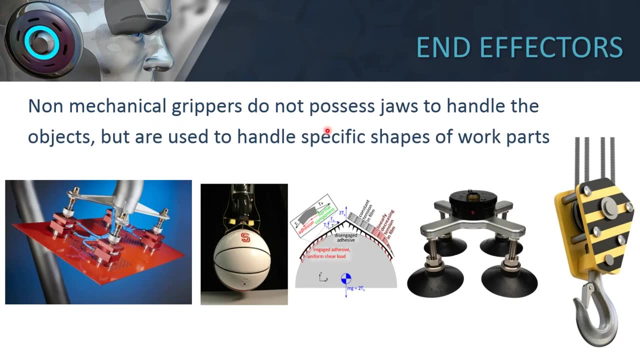 So likewise these mechanical grippers are used. The main function of the grippers is to grasp the object firmly in between the jaws. And there are certain non-mechanical grippers as well. They do not possess jaws to handle the objects. 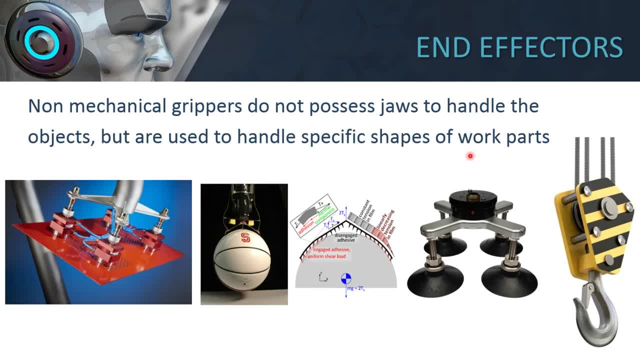 But they are used to handle specific shapes of a work part. They are So they are. So this magnetic gripper, This can be a magnetic gripper wherein the iron sheet, The sheet which contains iron, can be grasped firmly because of the magnetic action. 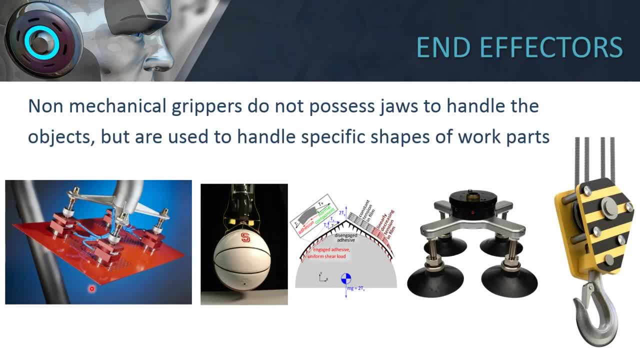 So when the switch is turned on, the magnetic force comes into picture, and then it grasps the sheet And then it can be moved to a particular location where that sheet has to be dropped. And then there is one more type of gripper, wherein that is called as adhesion type of gripper. 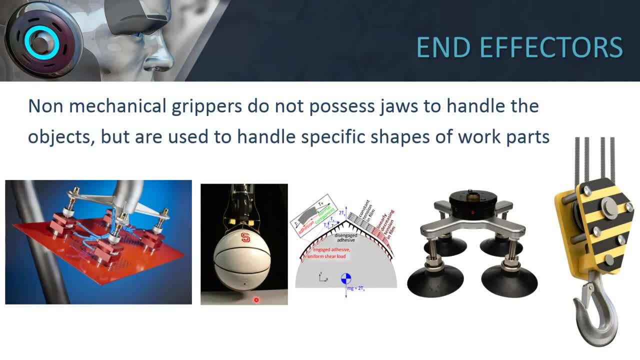 It is used to hold curved objects. So you can see the adhesion here. So this helps in holding the curved objects. There is one more non-mechanical gripper which is called as vacuum grippers. These vacuum grippers are operated by pneumatic cylinders. 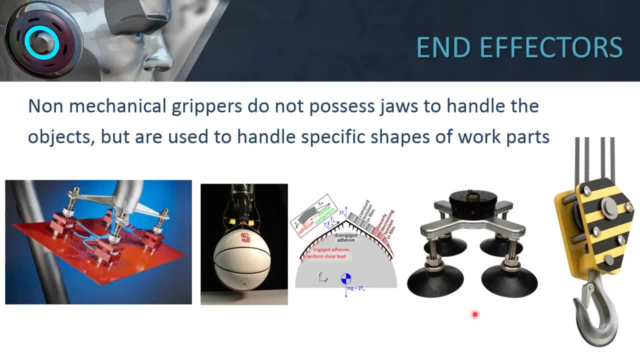 That is, by the help of the air compressors. What happens when the air compressor is switched on? There is vacuum created, There is suction cup. These are called as suction cups. When the vacuum is created, it grasps the objects And then it has taken to a different location. 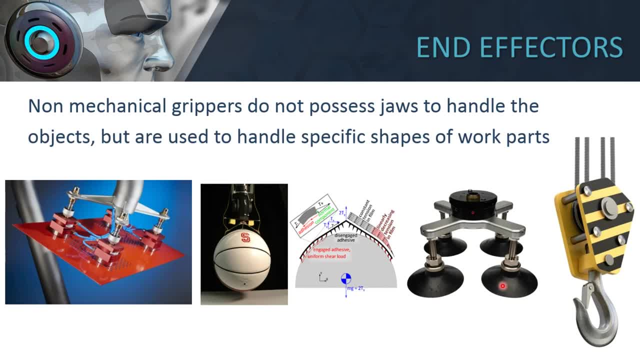 And then it is put at that particular location. Once the product or a material is dropped in that particular location, the air compressor, the flow of air is switched off And then these suction cups will be removed or it will be taken apart from the object. 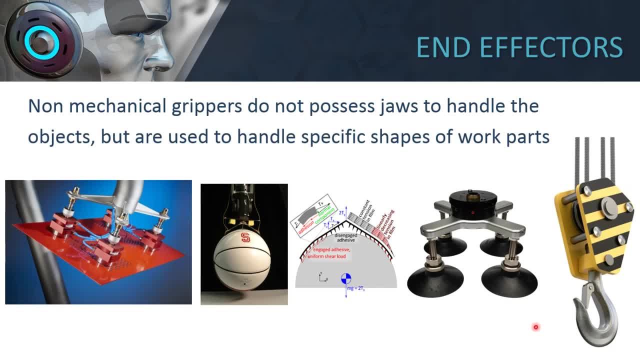 That is how you can use this non-mechanical gripper. And then one most commonly used type of non-mechanical gripper is the hooks You would have seen in the cranes, wherein the part is put across by a rope And then the rope is put into the hook. 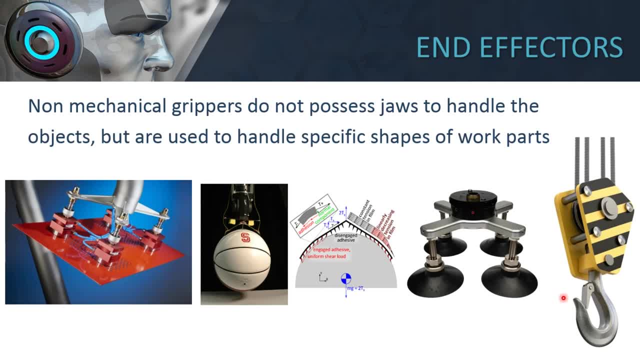 And then by this it can be lifted and then taken to a different location. So these are some of the non-mechanical grippers, what you can use in a robot or a crane or any other device Which will help you, Help grasping the objects and putting it into a different location. 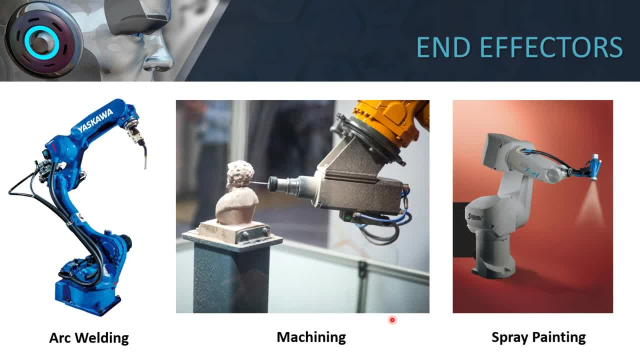 There are certain tools used as end effectors as well, And they can be the electrode holder as to perform the arc welding process. That electrode holder can be installed as the end effector. This is a arc welding machine, Everything else remaining the same.